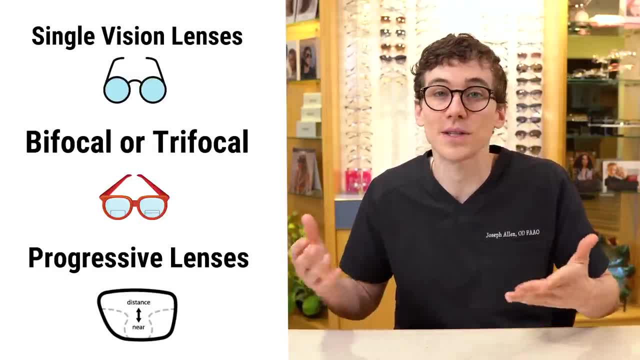 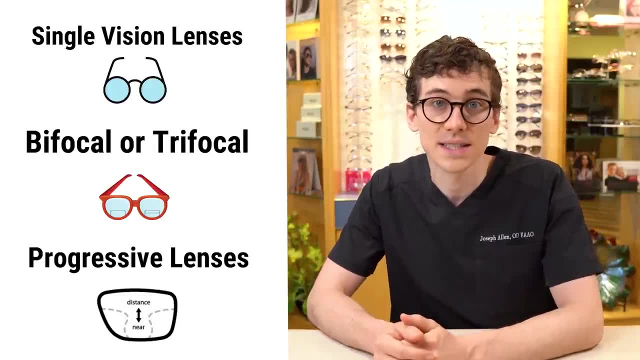 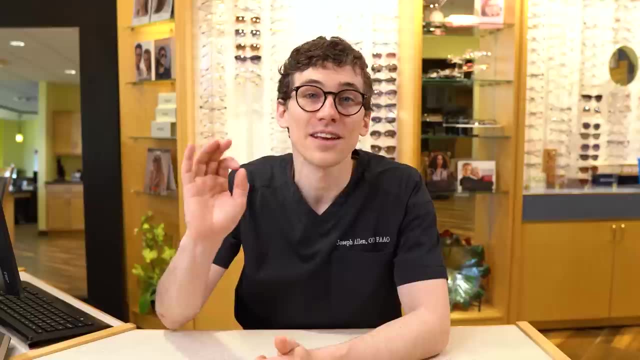 trifocal glasses for people who need distance and near simultaneously. And then you can have progressive lenses And, depending on your country, you may know them as varifocal lenses. Single vision distance lenses are pretty straightforward and are the standard glasses lens to help people see in the distance very well. So whether you are someone with 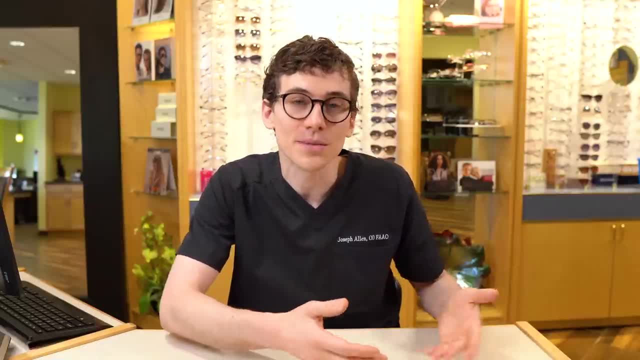 farsightedness, nearsightedness, or have astigmatism. these are probably the lenses that you're going to want to look for. So if you're looking for a lens that's going to be used for computer glasses, then you have. 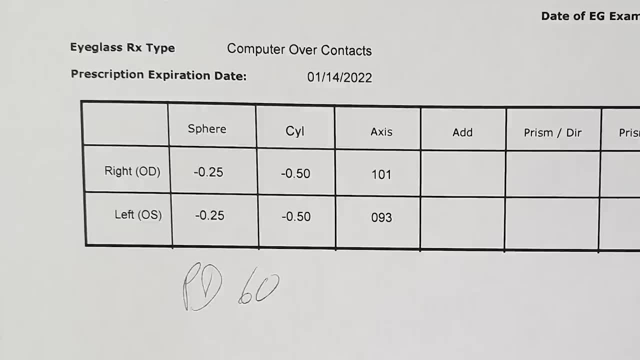 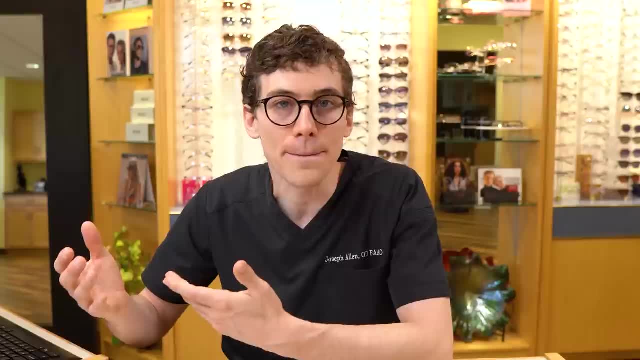 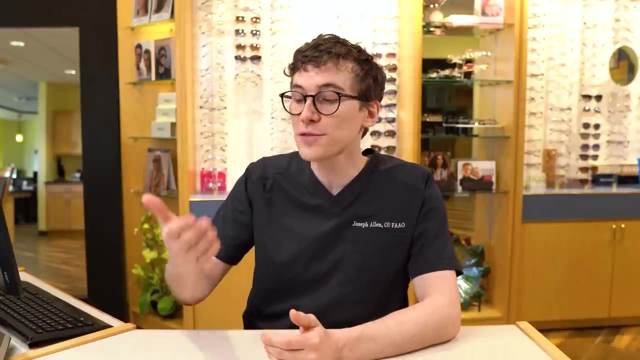 to have a bifocal lens If your glasses prescription also has an ad on there short for additional lenses, this is meant more for someone who needs something like a bifocal prescription, a trifocal or a progressive lens. Now single vision lenses can also be made just for reading. 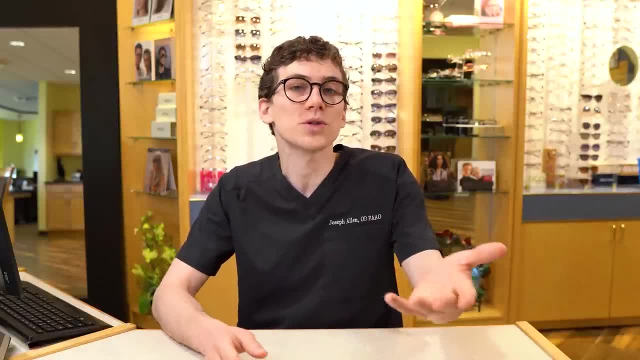 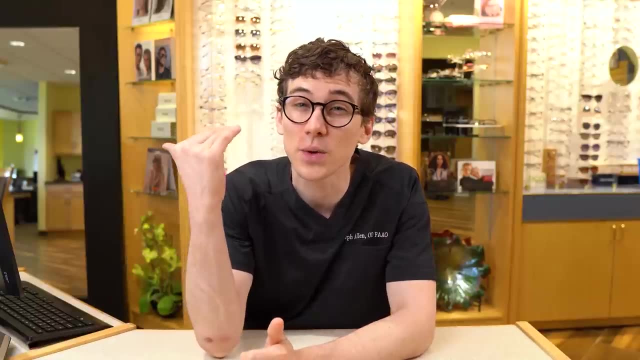 up close or being on something like a computer, And we call those near vision lenses or something like reading glasses or computer glasses. Bifocal glasses are the lenses that have that extra line going through the middle of the lens. So if you're looking for a lens that's going to be used for, 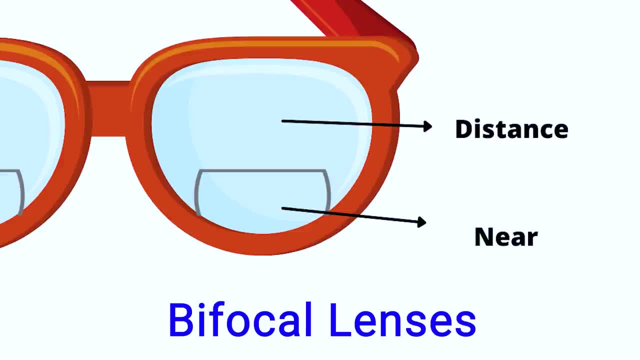 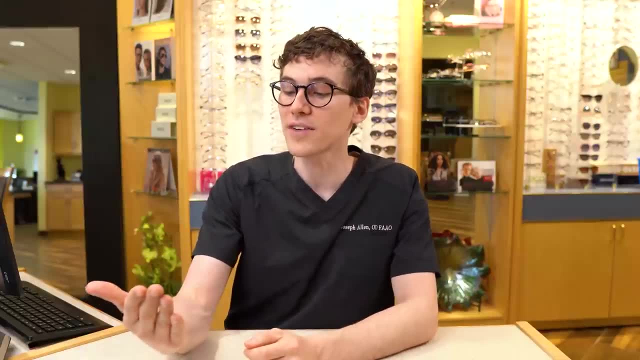 reading up close. that's essentially an additional magnifying lens that's attached on top of your distance vision prescription. That way you can see in the distance and look through the magnifying lens and see things up close. For some people who need more than just a distance and a reading, 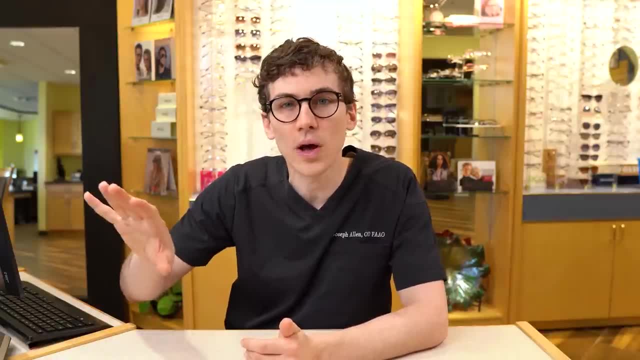 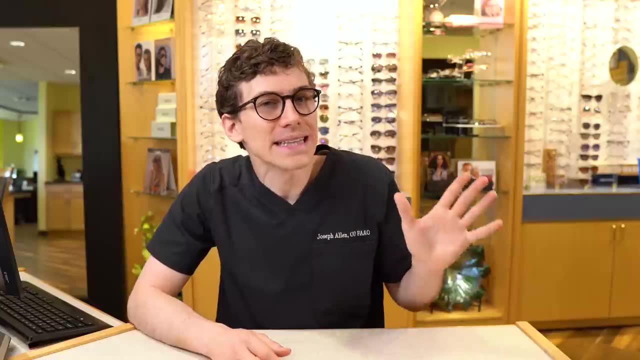 prescription but want to be able to see that intermediate zone as well. there is also a trifocal option that has an extra line on there. So you have three levels, but not everybody likes these two different designs for bifocals or trifocals. 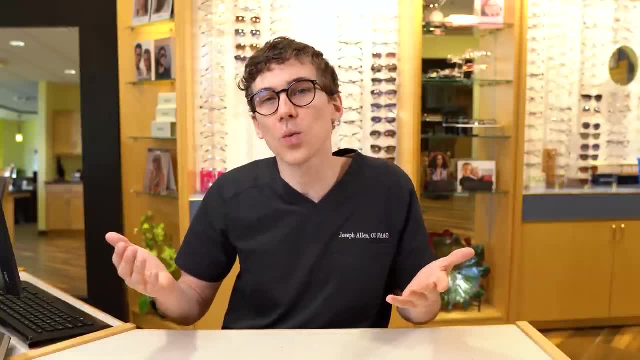 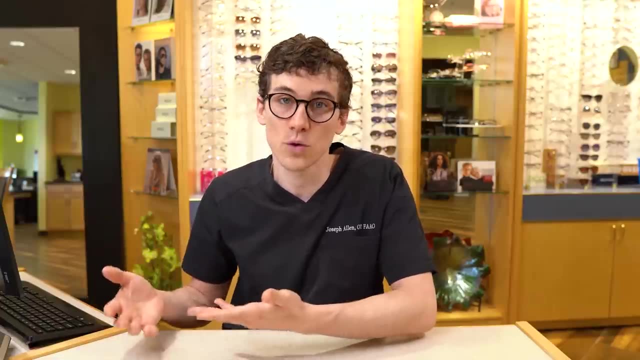 Because that line makes them either look older or the line gets in the way of their vision, And so most people nowadays will end up reaching for something called a progressive lens or a very focal lens. Progressive or very focal lenses are eyeglasses, lenses like a bifocal or 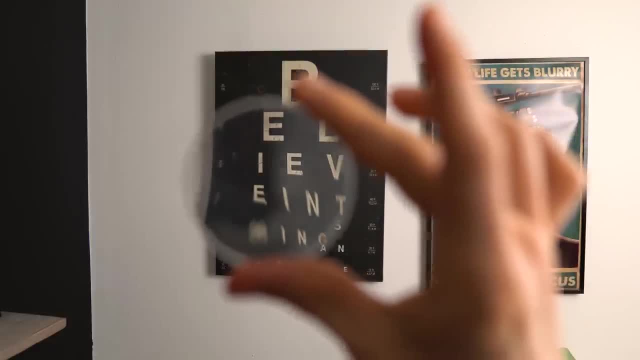 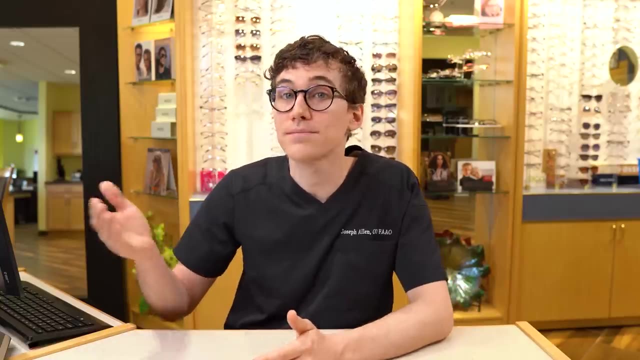 a trifocal, But instead of just having like two or three segments, it's like having 25 segments where the lenses are all blended together. That's why a lot of people will call them no line bifocals, Because again, you cannot see the line. 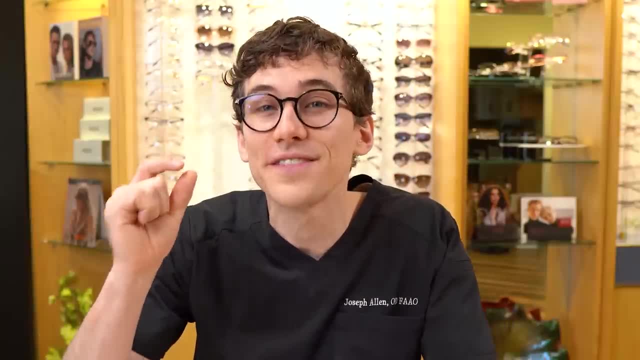 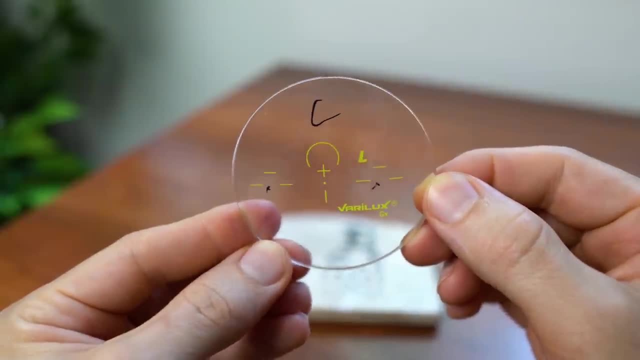 Even the glasses I'm wearing right now have a very slight reading prescription at the bottom, but it's all blended together and you can't tell. But these lenses are often ideal because they not just let you see in the distance and up close, but they give you many different levels of range. 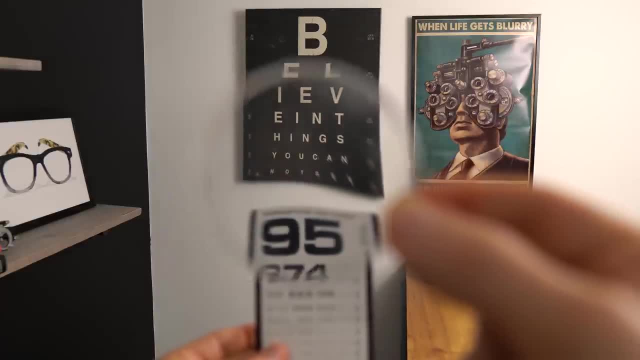 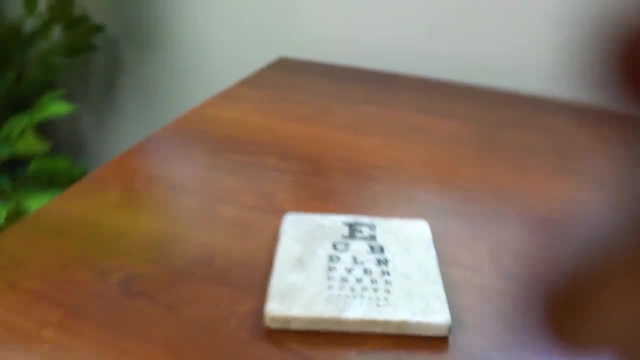 for reading, things like on a computer, a dashboard and other things. Now there is a lot to be said about progressive lenses. One brand of lens is not the same as another and they give you completely different visual experiences. And we do have a video coming. 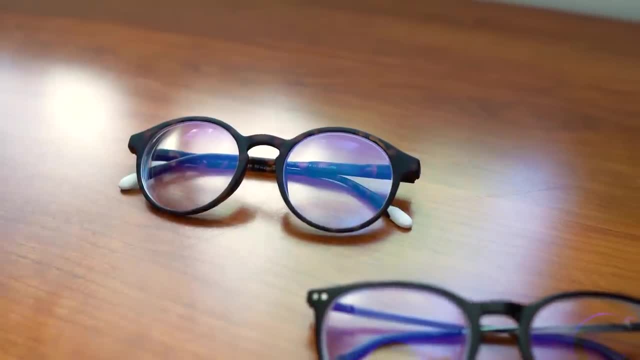 out soon on progressive lenses, but I'm not going to go into that right now. So if you're interested, you can go ahead and check it out And I'll see you in the next video. But now that we've gone over different lens design options, let's now go over different. 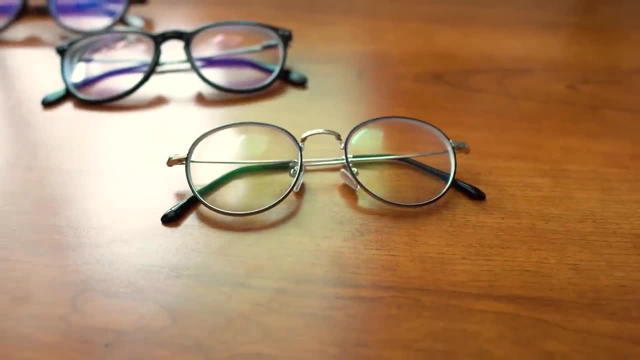 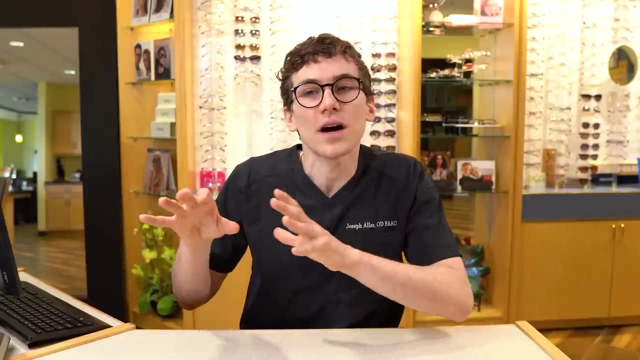 lens materials, because there are some lens materials that have better advantages over others And because there are many different options and they can get a little confusing if you're not in this optical world, a lot of glasses shops like the one we're at here. 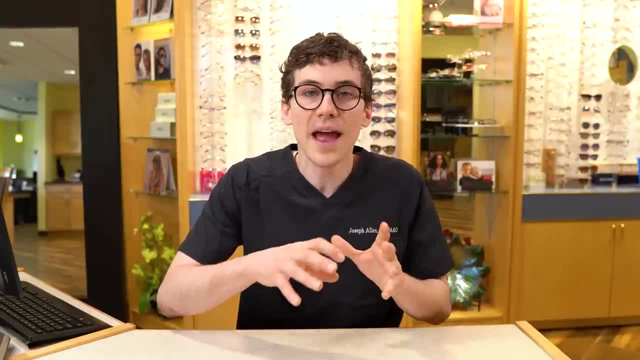 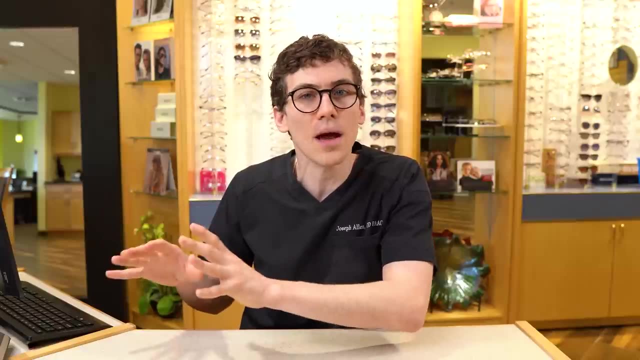 as well as a lot of online glasses websites. they'll have the lenses broken down into what are called lens packages, breaking down from more affordable, cheaper lens options all the way up to premium lens options, which you will see better out of and have a better visual experience. but 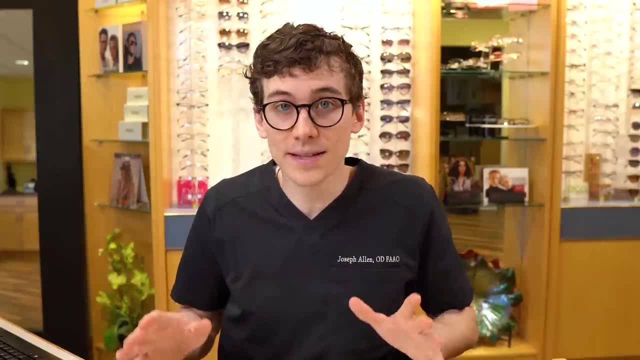 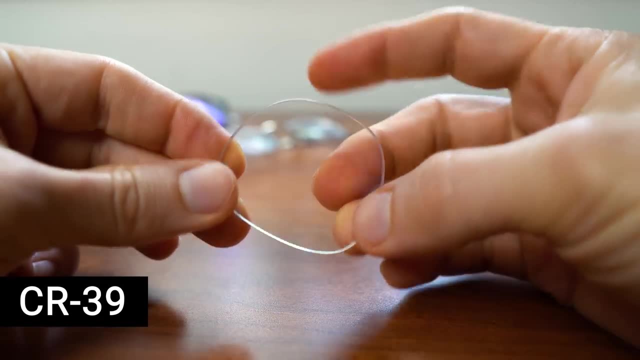 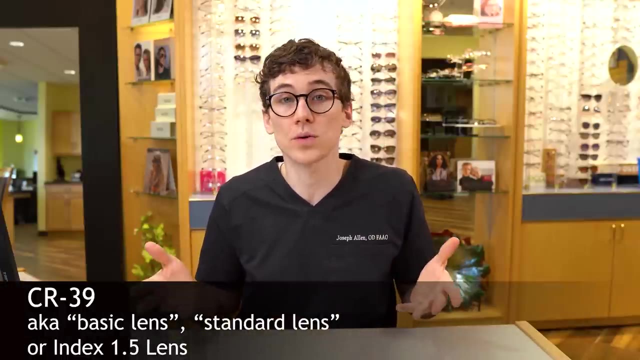 they're usually more costly. The basic thing that you need to know about glasses lenses is this: The most standard glasses lens that is used these days is, in fact, a plastic called CR39.. It is often referred to as a basic lens or a standard lens, or also known as a index 1.5 lens. CR39 is a great 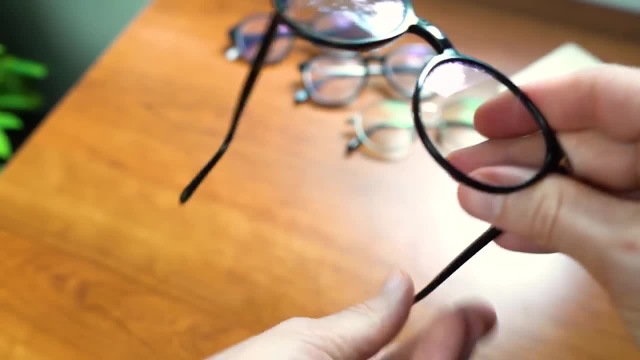 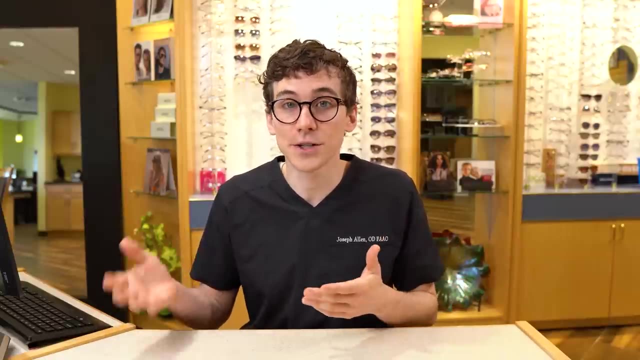 lens material. It has a lot of different options, but it's not the only one that's used. It's also excellent optical quality. it is light and it is very affordable, And for most companies this is just the standard lens that they are using, but then they offer upgraded materials from the CR39. 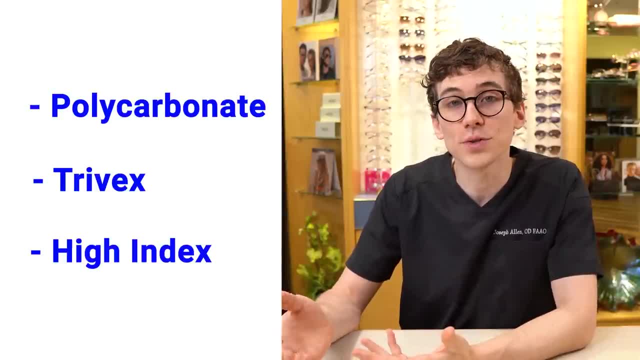 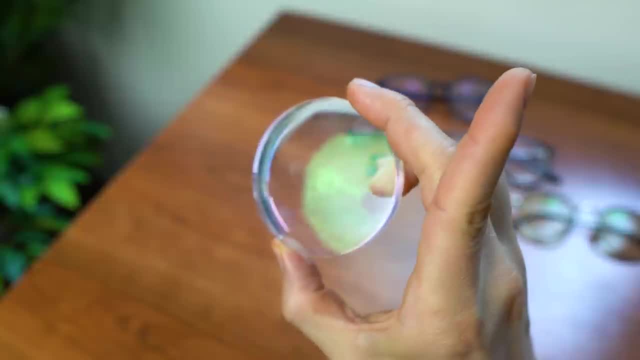 lens And most often the lens materials that you'll have options to include what are called polycarbonate trivex and what are called high index lenses. Polycarbonate lenses or polycarb lenses are a soft plastic type of material. Now, because of the high index lenses, they're not 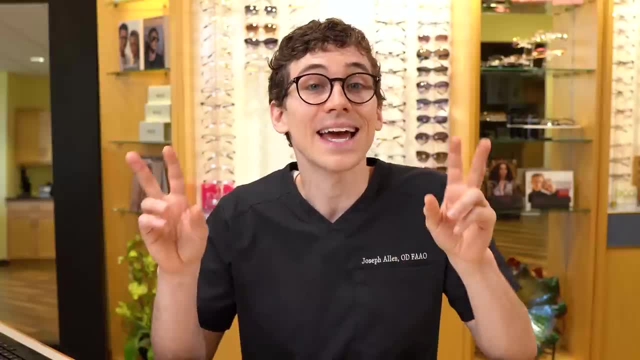 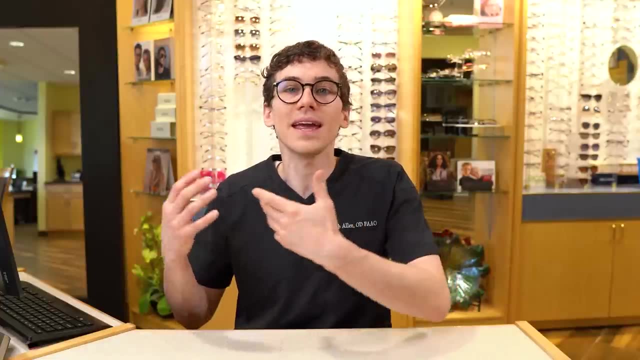 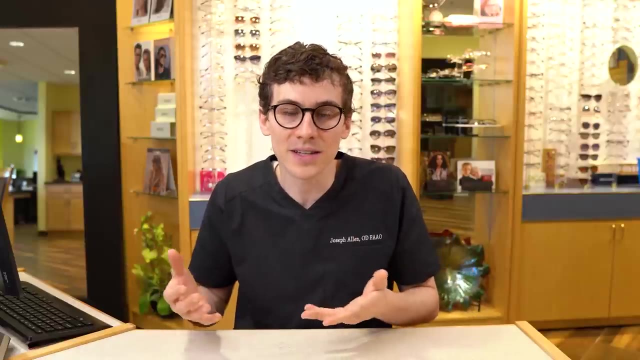 technically shatter proof, but they are more shatter resistant, which is usually recommended for somebody who is in, like a construction job, high risk for any sort of eye injury, or for children, who are just more prone to accidents and breaking their glasses. 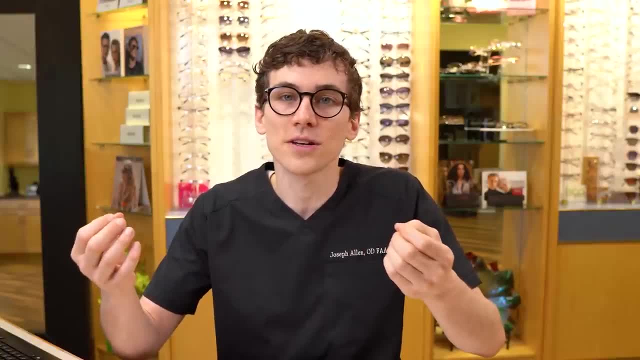 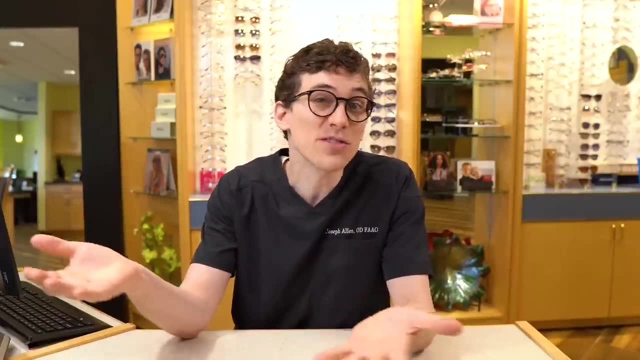 because we don't want the lenses to shatter And then you get the shards of glass or hard plastic into the eye. Polycarb lenses also offer an innate UV light protection of about 90%, And that's because they're made with glasses lenses And because of the way they're made with. 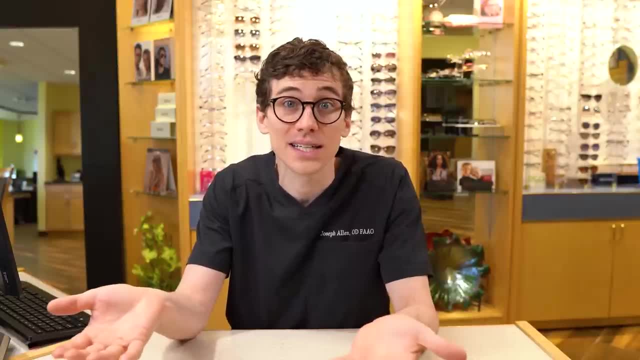 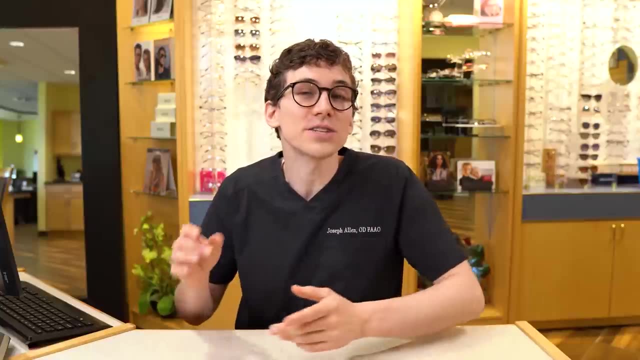 glasses lenses. they have about 99 to about 100% protection from sunlight And they also are usually thinner and lighter than CR39 plastic. However, polycarbonate does have a rather low Abbey value, which means that they'll have more aberrations looking from the sides of the lenses. 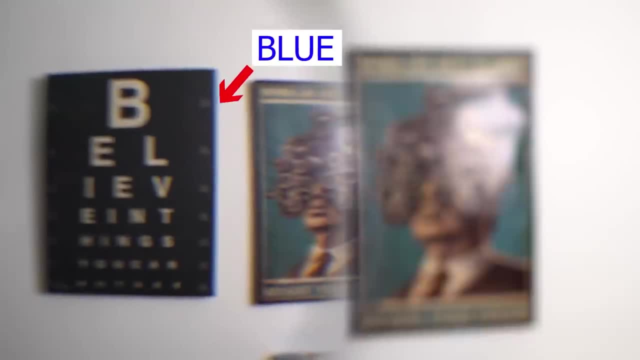 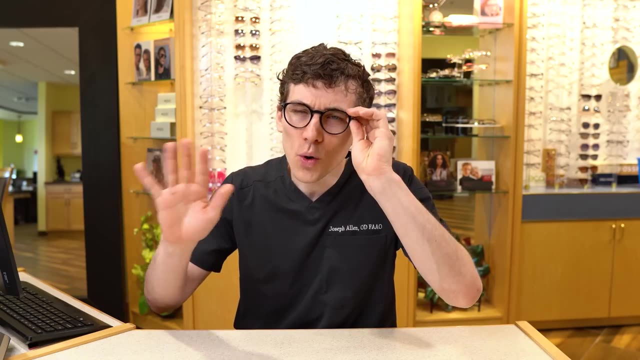 So if you have a really high prescription and you look off to the side of a polycarb lens, you might see these color distortions, such as yellow or blue, kind of fading off to the distance. Most people don't notice those sort of color distortions, but I have. 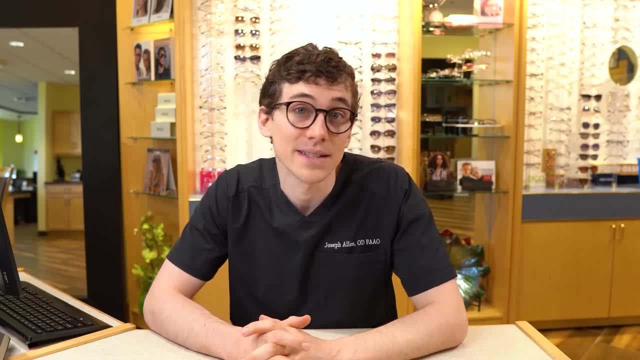 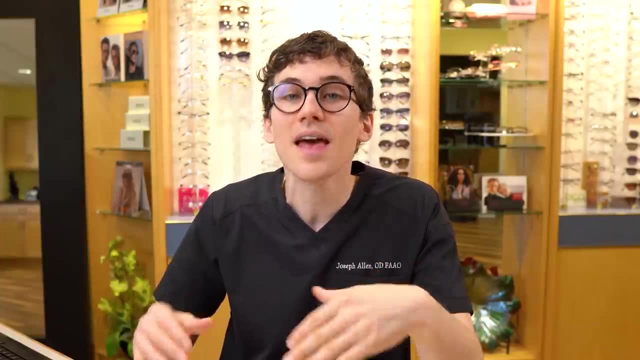 had a few people on this channel ask about that, So I just wanted to shed some light on the subject. The only other thing about polycarbonate lenses that you should watch out for is that, even though they are more shatter resistant, they are a softer plastic, and so 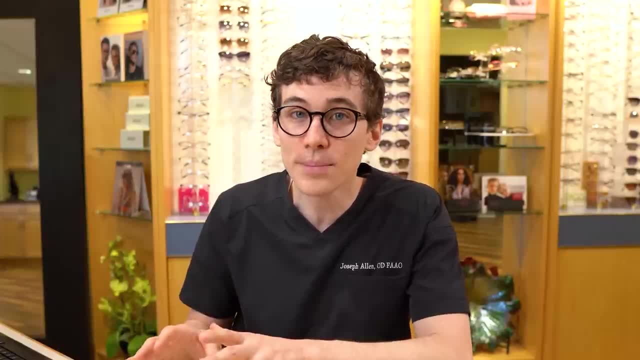 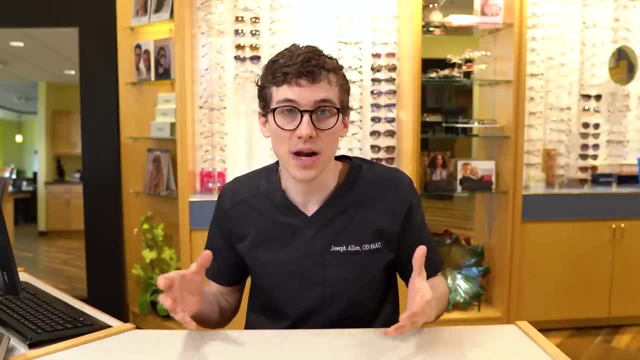 they are usually easier to scratch. So if you're getting a polycarbonate lens, highly recommend you get some sort of anti-scratch coating put on those lenses. And then we have a lens called Trivex. Now Trivex is a registered trademarked material that is similar to polycarbonate in that it is similar to polycarbonate in that it is similar to polycarbonate in that it is. 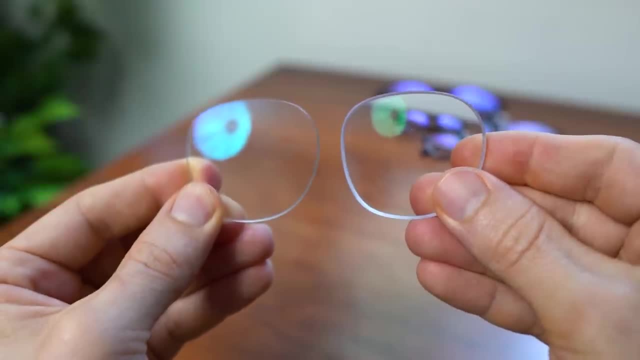 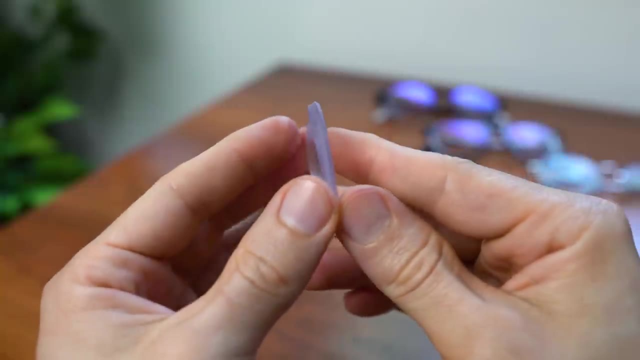 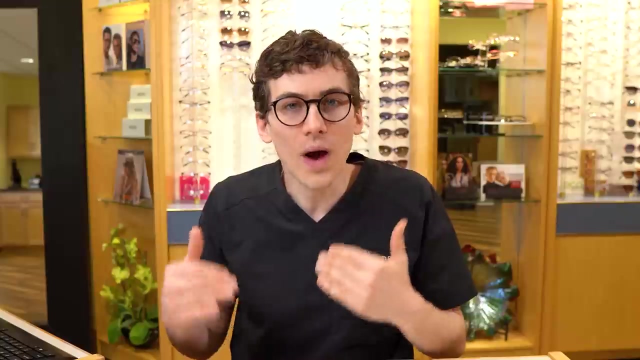 about 10 times stronger or impact resistant than a standard CR39 lens. It does have some advantages over polycarbonate in that it is lighter and has better optical quality than polycarb and it has less aberrations than the polycarbonate lens, So I personally like to think of it as an upgraded. 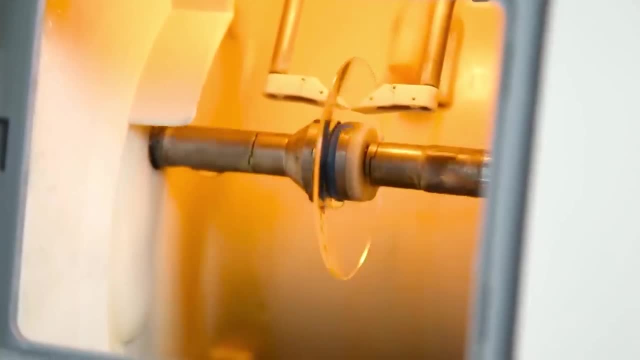 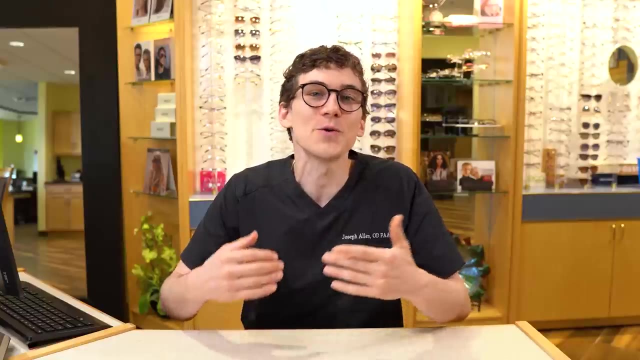 kind of better version of polycarbonate Plus. a fun fact is that when you're grinding and making these lenses for glasses, Trivex lenses smell bad. So if you want to punish the person who is making your glasses lenses, go ahead and order Trivex lenses. 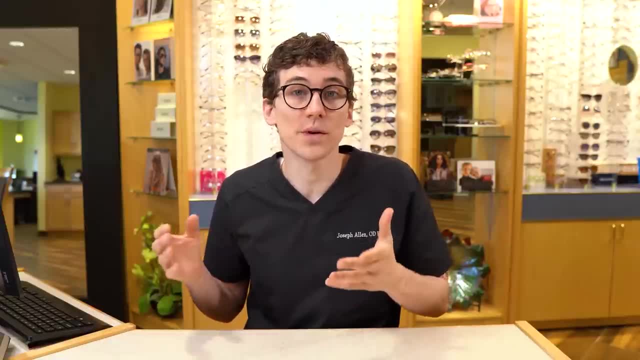 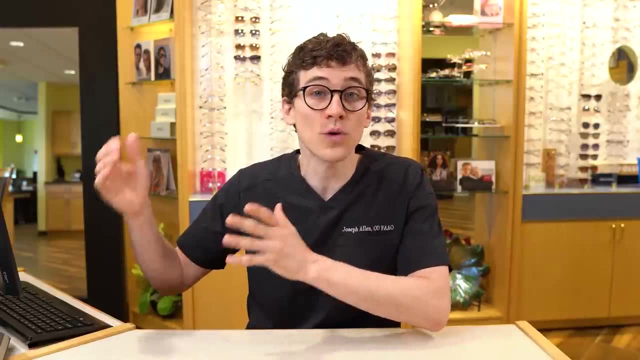 Now, high index lenses refers to the lens's ability to refract light, Meaning that if you have a higher index, such as a 1.69 lens or a 1.74 lens, you need less lens material to get the same effect.